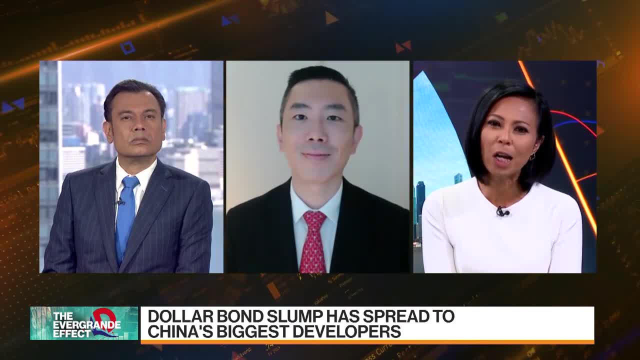 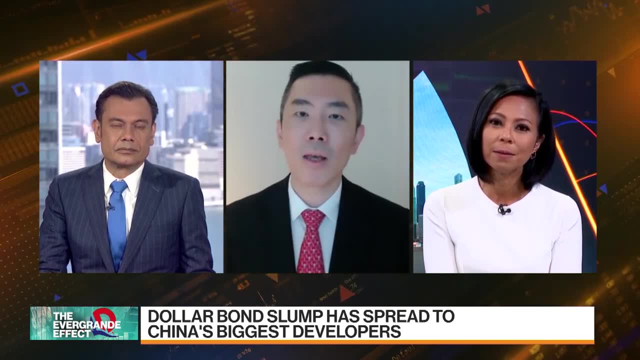 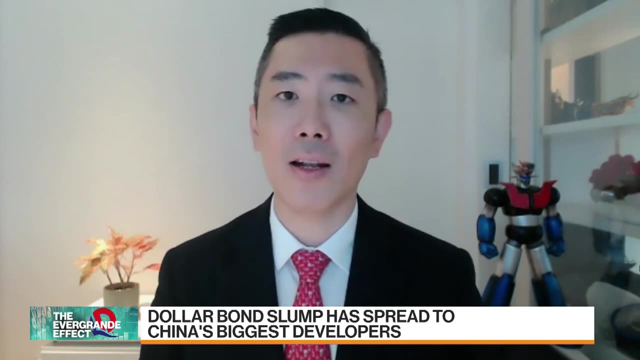 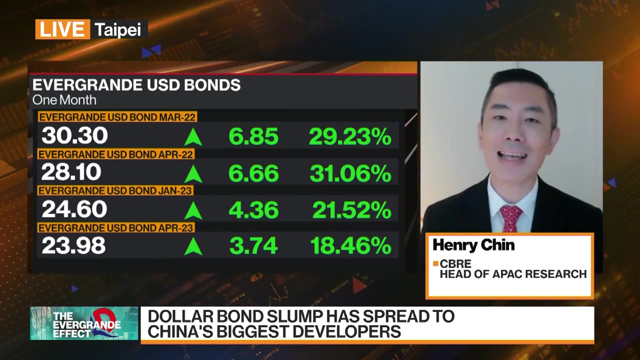 junk bonds have yielded the surge more than 20 percent right now, making it even more difficult for companies to pay back. Yeah, you are right, I think for developers- while we are working for our clients, we look at the developers. There's a few viable options. It's number one: looking at the underlying asset and those land bank. Some of the land bank they are holding is quite valuable. So what we are seeing is they are going to dispose of those assets to enhance the balance sheet, to pay off the debt And you can see the money: monetary easing. 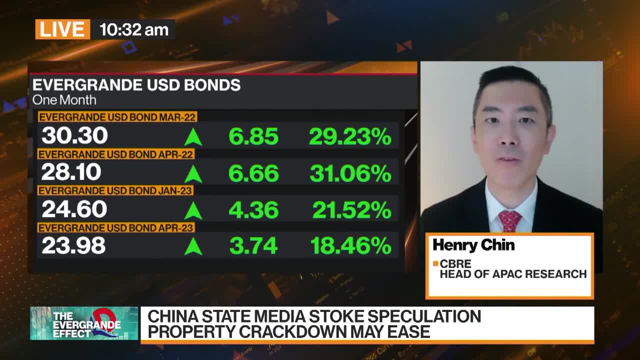 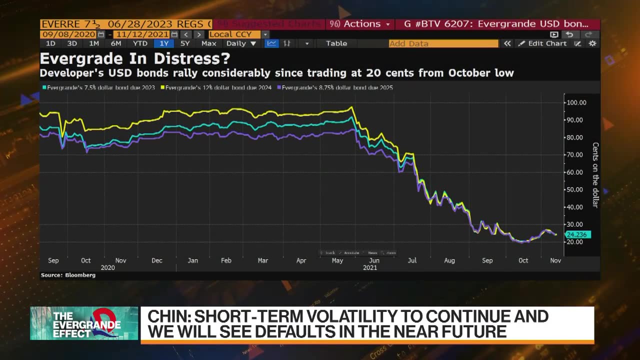 policy coming, introduced by the government, potentially going to provide more liquidity to those healthier developers. So, in my mind, in 2022 we are expecting to see some consolidation in a residential property developer sectors. So MMA, in my mind, is coming to the car. We know that China's growth going forward will be boosted by innovation, will be boosted by tech. Give us a sense of how this will impact demand for, perhaps commercial real estate. 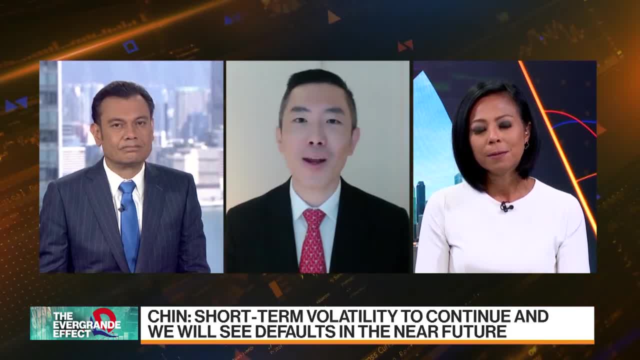 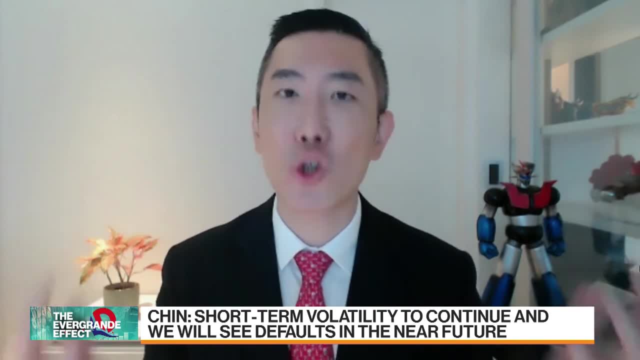 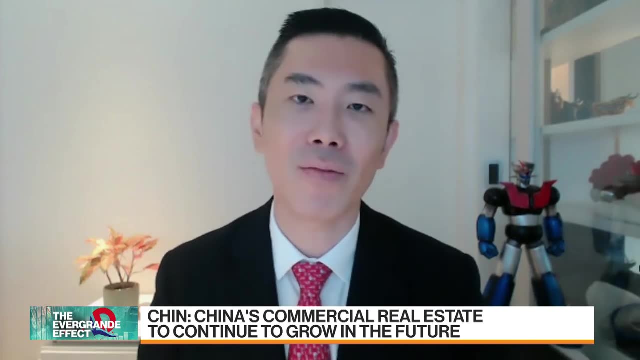 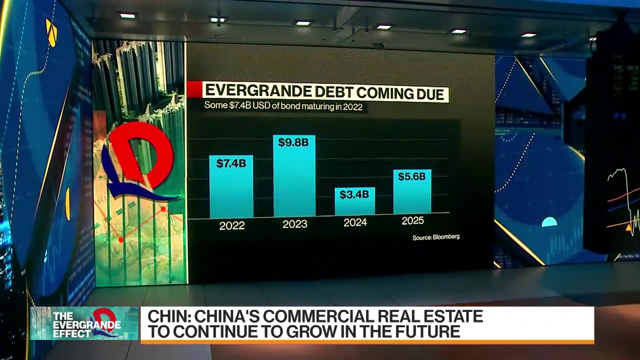 What assumptions are you making? I think commercial real estate market is in the early stages for booming. I have to say, if you look at a US commercial real estate market size, it was 11 trillion US dollars. China, being the second biggest economy, is only 3.8 trillion, A third of the size of the US. as a result that, we are seeing more and more investors are tapping into the commercial spaces, particularly logistic tech, cost storages and data centers, as well as life sciences. All of these are 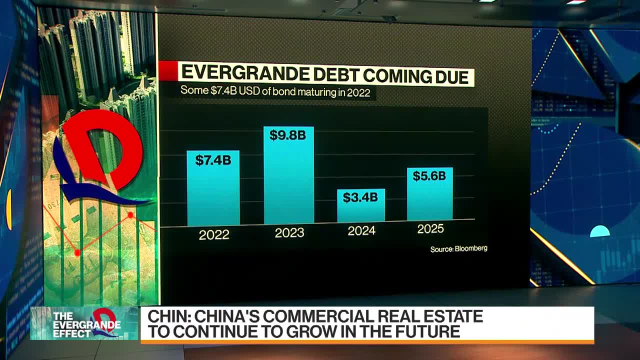 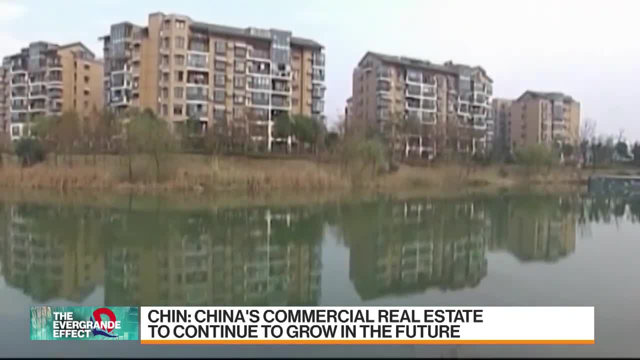 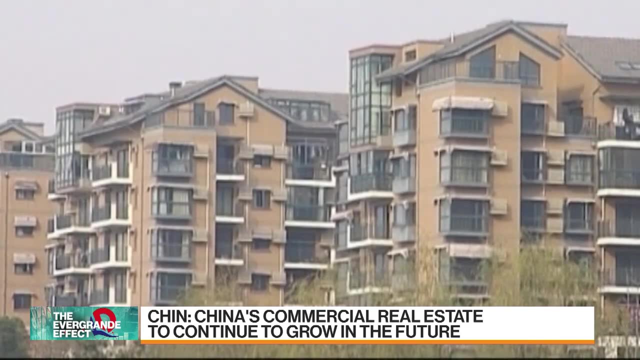 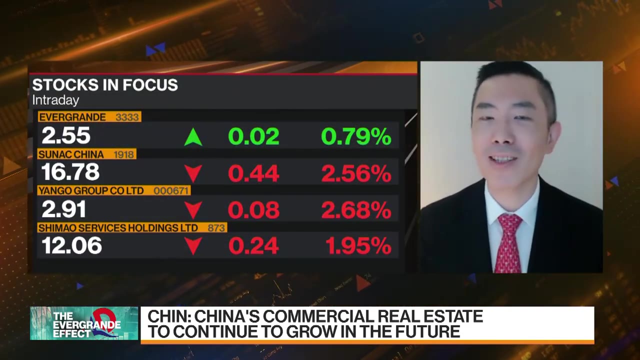 those investors are tapping into these spaces. I think residential growth is coming to the end, But we are very confident to see the growth coming from the commercial real estate spaces for foreign investors looking to put the money in China's real estate sector. Where should they be putting the money, Henry? I have to say demographic really is important. Follow government policies, even crucial. 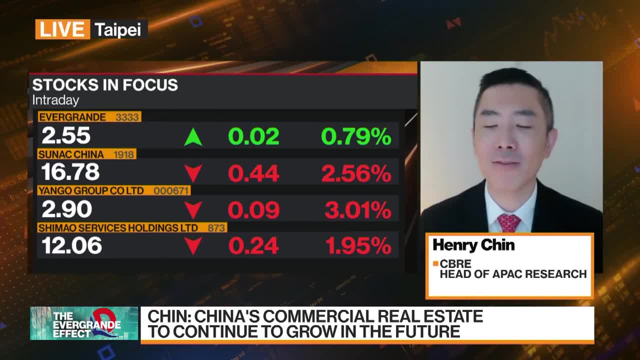 for investing into China. I think for China we're pretty much like a four class at a Beijing class, at a Shanghai class, at a greater bay plus and Chengdu class, at a loss of four classes. It's going to be a lot more powerful, a lot more prosperity. I'm going forward.